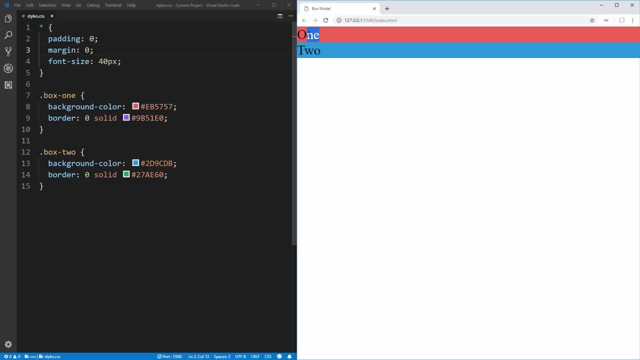 If you do nothing to a box at all, the content of the box is just going to fill up the space inside of the box and the box will be no larger than the content. But if you start adding different things to the box, then you can start to expand the. 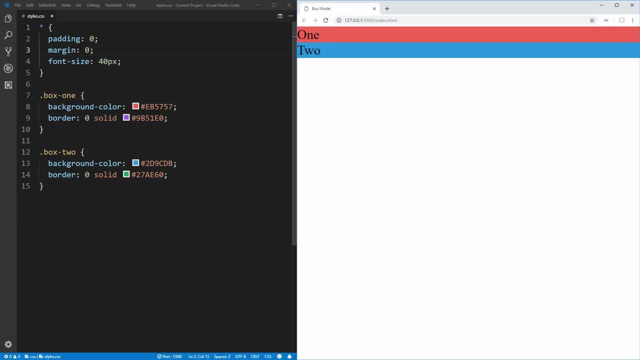 size of your box. So, for example, one of the easiest ways to make your box bigger is to use padding. So let's add padding to this element. We'll just add 20 pixels to box one And if we save that, you see that our box has increased by 20 pixels on all sides. 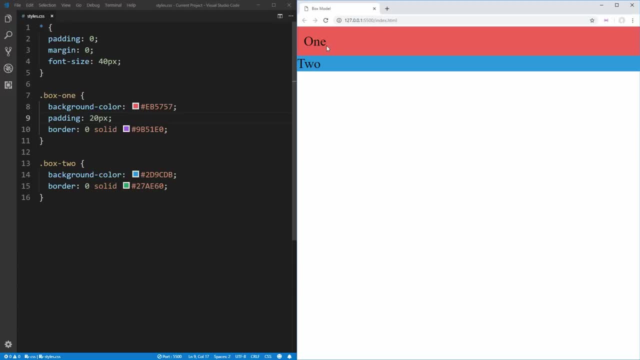 Everything is pushed away from this one text by 20 pixels, And that is because padding occurs inside of the background of the element. It occurs inside the border, essentially, and it goes around the content of the element. So the content is the very most inside thing in the box model. 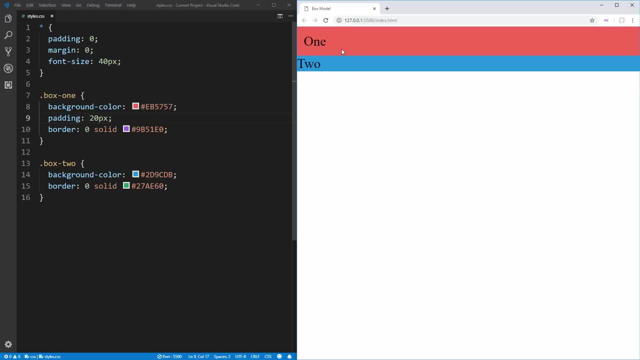 Then we have padding next, which will include the background color of an element. So most of the time we're going to add padding to this element. The buttons in CSS are styled using padding so that the background of the button becomes wider than the actual text of the button itself. 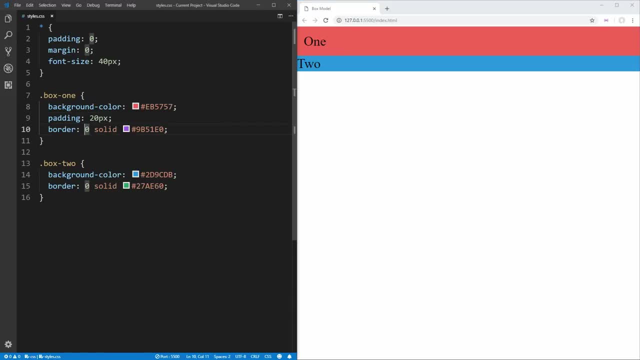 The next thing we can talk about is the border of an element. So if we change this border size here to also be 20 pixels, it's going to be a nice purple color. We can see that we get this nice purple border that goes around the padding of our element. 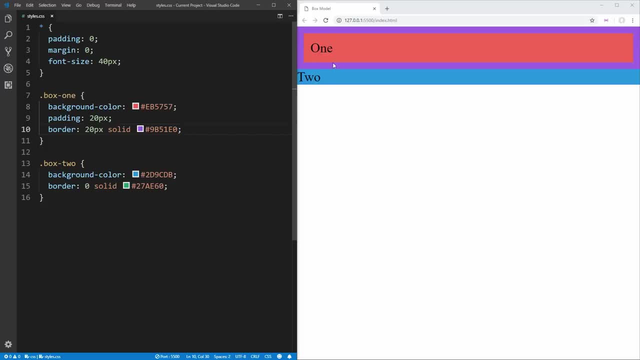 So we have our 20 pixels of padding around our content and then we have 20 pixels of border around the padding which is around our content, And the very last thing that we can have on our element is margin. So if we just add 20 pixels of margin to our element, you can see that is spacing on the 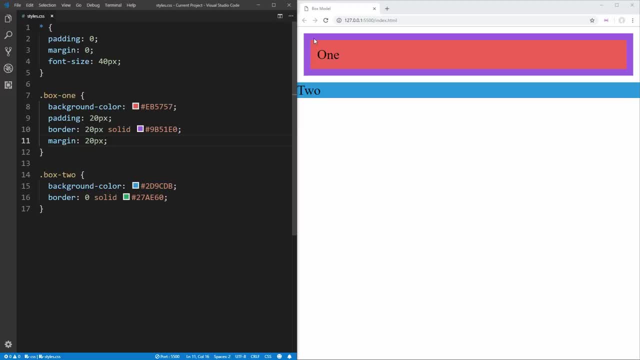 outside of our border, and margin is what we usually use to space two elements apart from each other. Padding is mostly used to add background to an element to make it go around the content, and margin is specifically to go around two different items to make them spaced apart. 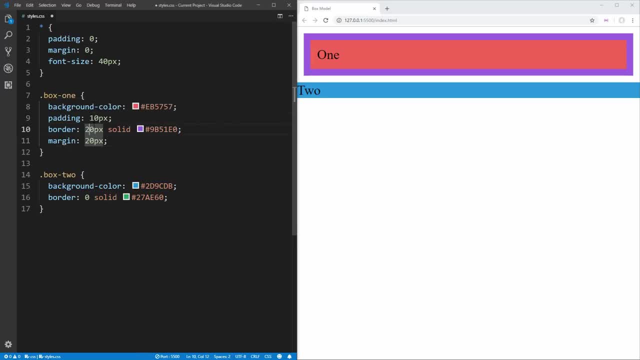 from each other. So now let's change these values so that we can see the difference between them. So we'll just make them all completely different. If we say that you see that we now get this element here, And if we right click on this, we can see that we now have this element here. 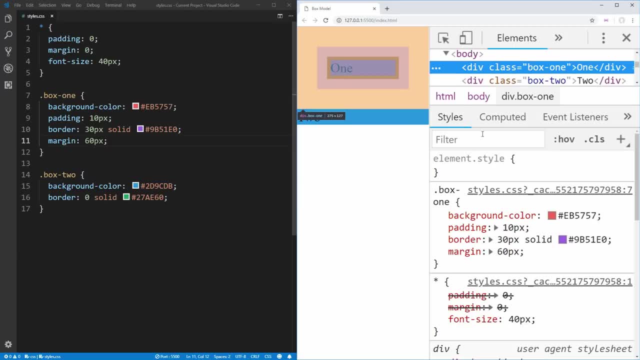 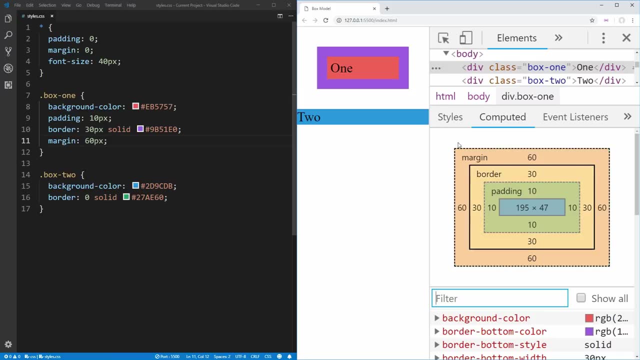 And if we right click on this and go down to inspect, we can see the different styles. So if we click on this computed tab, we can see, using the Chrome DevTools, all the different sections of the box model. This rectangle right here is the box model and on the inside, this blue section, this 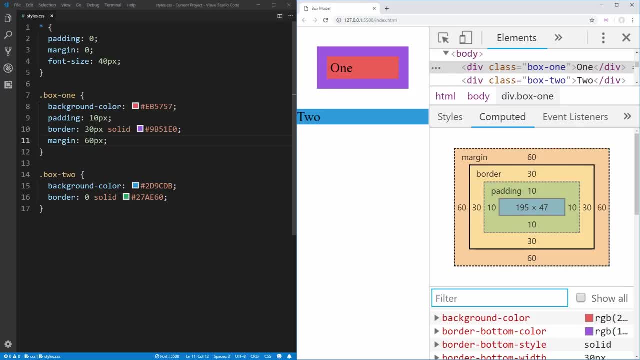 is the actual content of our box. As you can see, it's the thing that surrounds the one. when we highlight it, You can see that it is just the very intersection content of our box. We can specify distinct sizes of our content using the height and width property. 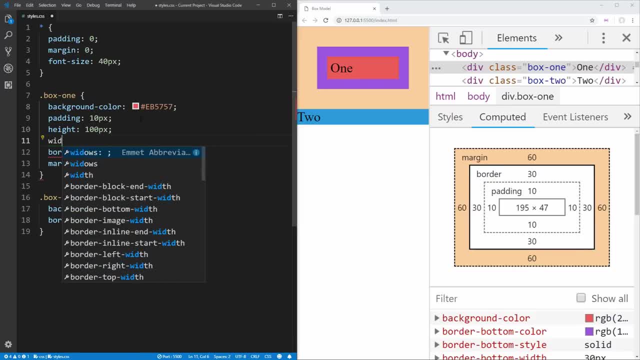 The height here of 100 pixels and we set a width of 100 pixels. You can see that we now have a 100 by 100 square And this blue section is that 100 by 100.. Next we have padding, which is this greenish color that you can see. 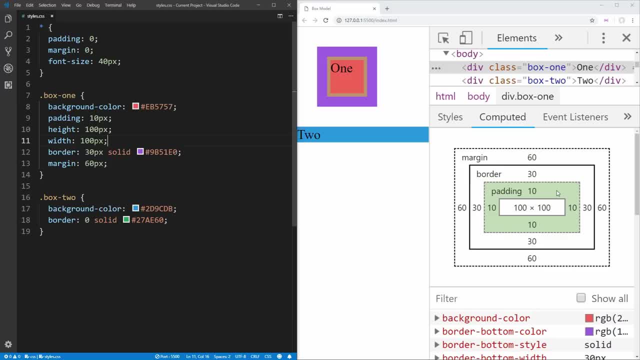 And, as you can see, it's 10 pixels. that goes directly around the word one. You can see it just barely touches it. So this is just around the content And it also goes outside of that height and width that we've defined. 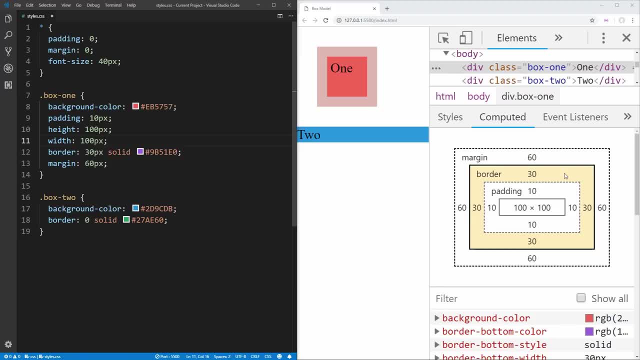 Next is that purple border Which we can see by hovering over here, And it's around the padding, as I've said. And then, lastly, this margin which goes around the element itself on the outside of the border, And it's used to break apart two elements from each other. 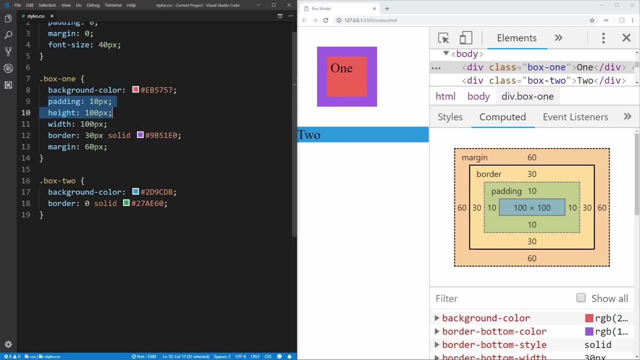 So now let's do a similar thing to box number two. We'll actually just copy all this code down to box number two, We'll paste it here, We'll remove the margin for now And we'll save that. And we see that our box number two is showing up right here. 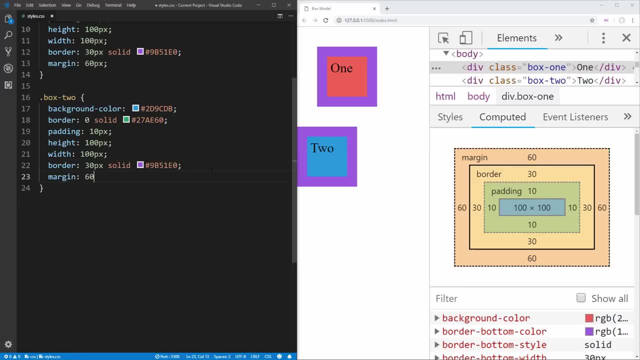 And now, if we add a margin of 60 pixels to the spot, This box, You would think that the box would end up moving down because it needs to move 60 pixels further away from box one. But if we save that, you see that it doesn't actually move further away. 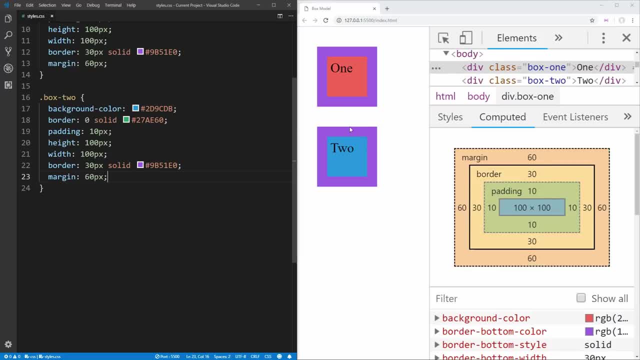 And that this 60 pixel margin is the same between these two elements. There's only 60 pixels here and not 120 like you would expect, And that's because in the box model margin actually collapses between two elements that are next to each other. 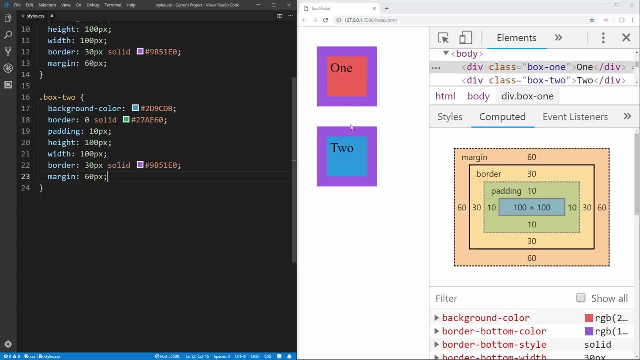 So, since these elements are right next to each other and they both share a margin, whichever margin is the largest is the one that will be used. So if we change this to 70,, for example, they now have 70 pixels of margin between them. 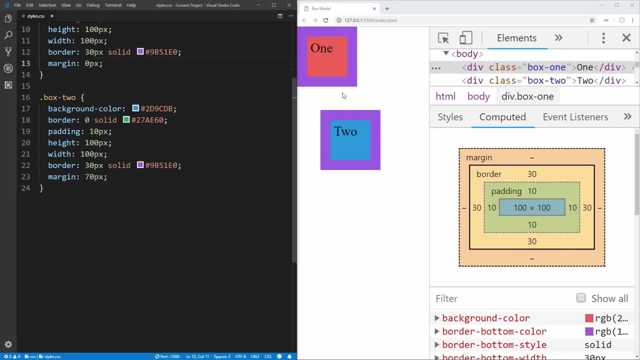 And even if we decrease this down to zero, you can see that it still has that 70 pixels of margin between them. But if we make this 100, it now has 100 between these two elements And you can see that by just hovering over here. we see that 100 margin. 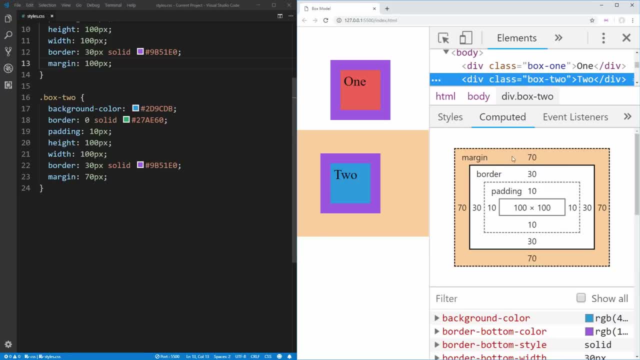 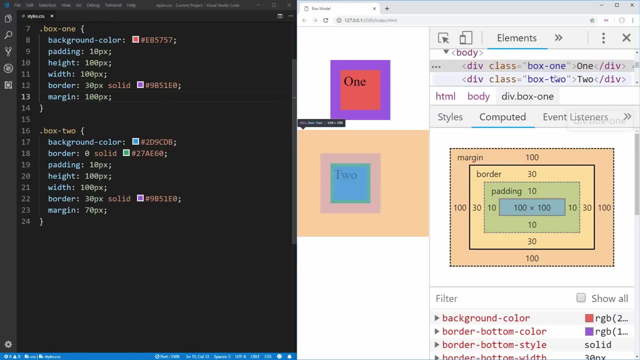 And if we select box two, it has that 70 margin but only 30 more between here and here, because this is a 100 margin between the elements. Another thing to note? Okay, Another thing to note is that if we hover over box one here, you can see down in the 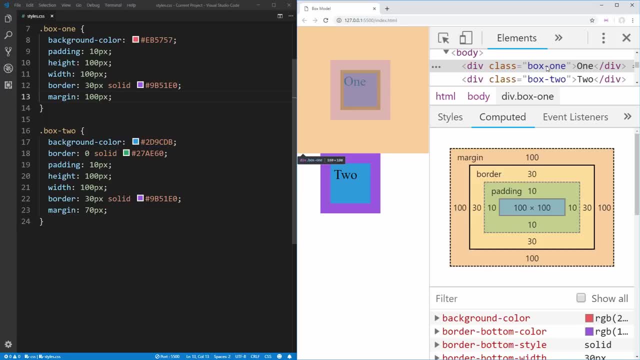 bottom left it says that the height and width is 180 by 180, but we actually defined our height and width to be 100 by 100. And that's because by default in the box model to get the height of an element, it adds together. 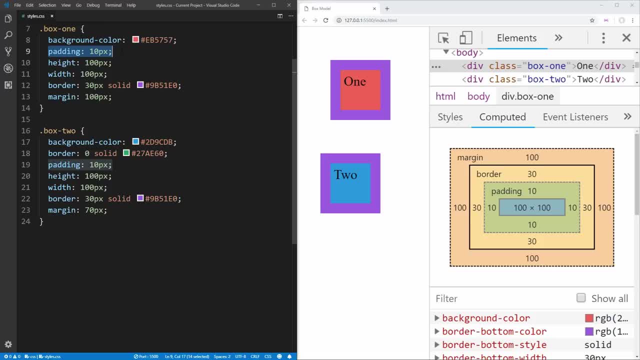 the height, plus it adds together the padding on the top and bottom. So in our case 10 on the top, 10 on the bottom would be 20.. So we're at 120,. does the same thing with the border on the top and the bottom. 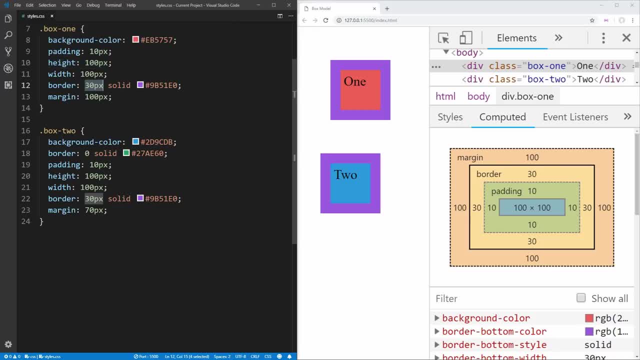 So we have 30 top bottom, which would make it 60. So now we're at 180 right here, And that's how we get 120. So we're at 180, as the height margin doesn't account into the height of an actual element. 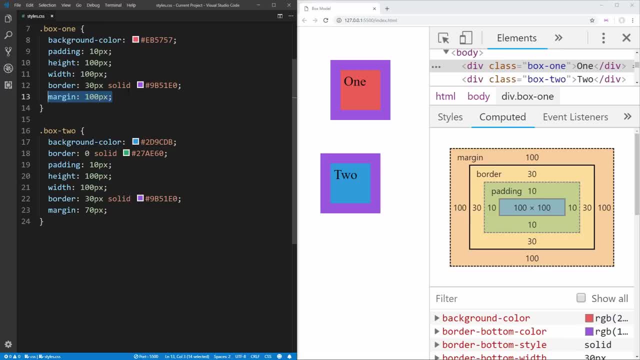 for sizing using CSS by default, But if we wanted to change this so that our height and width right here are the actual height and width of our element, what we would need to use is we need to change the box sizing of our element to be border box. 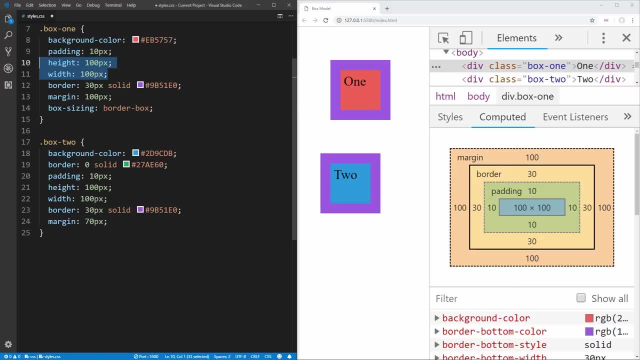 And what border box does is it makes this height and width account for the padding and the margin, or the padding and the border of our element. So let's change this border down to 20 pixels So it's a little bit smaller. And if you save that, you see that if we go to our box number one, our content section, 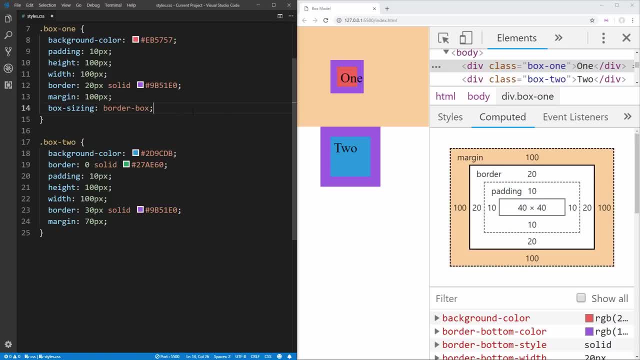 is only 40 by 40.. In the other example, without this border box- here you can see it's the height and width 100 by 100. But when we use border box, the actual size of the content gets subtracted out from the. 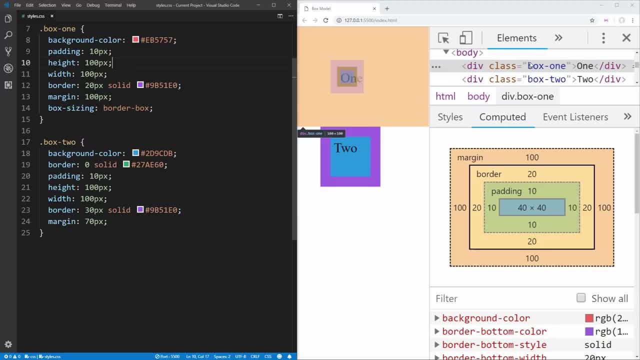 border and the padding, so that when we hover over this, you see, our actual element is 100 by 100.. Instead of adding all of these, it just uses this height and this width and the border and padding, So we can cut into that height and width. 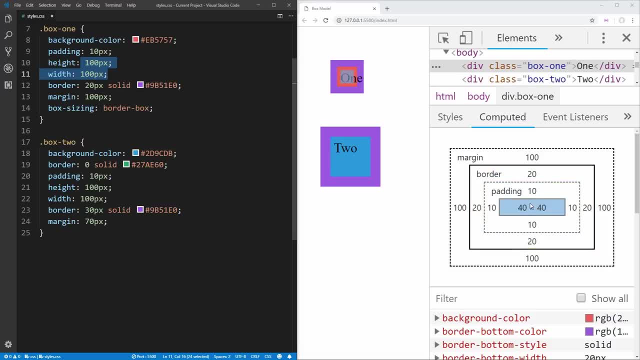 As you can see, our padding is still there and our border is still there, but the actual content of our element was shrunk down to be 40 by 40, so that the overall element, everything inside the border, is a total of 100 pixels instead of being 180.